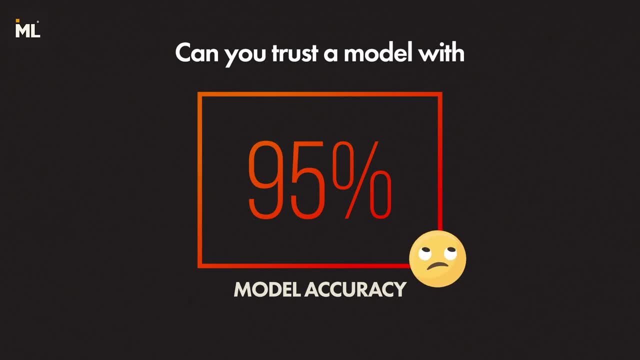 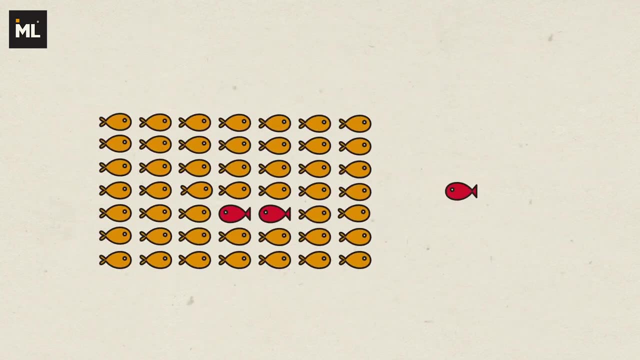 trust them? The answer is no. Well, here is an example. Assuming we have a model simply labels almost every fish as red fish and yellow fish and we want to identify the red fish among them. The answer is no. Given majority of the fish are yellow fish. the model can easily achieve 95%. 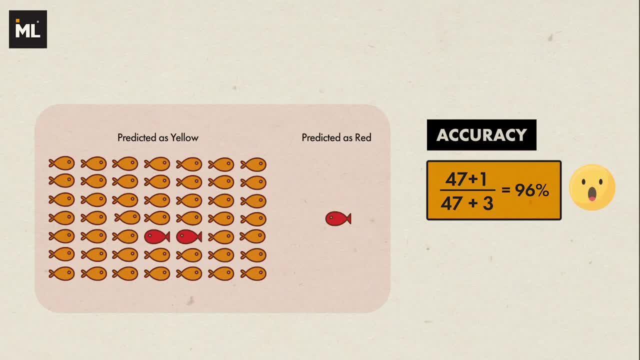 overall accuracy. Intuitively, we know that claiming almost all the fish are yellow fish is not helpful and we should focus on identifying the red fish, which is the positive class. Then the question is: how do we find a matrix to achieve this goal? 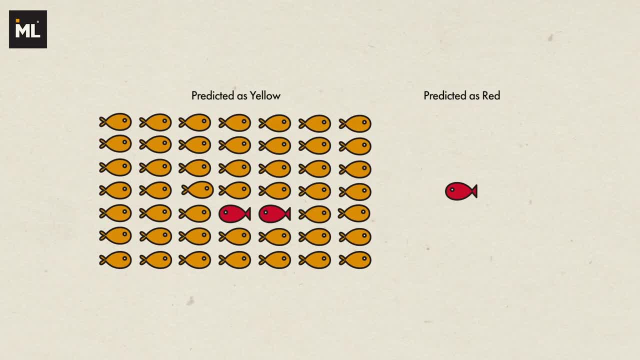 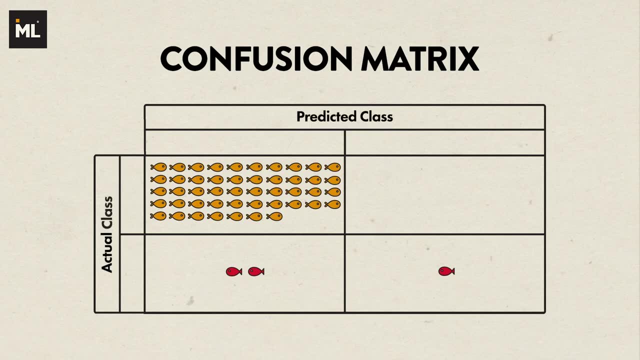 Now is the time to introduce Confucian matrix. In this matrix the columns correspond to what the matrix is. The red matrix is the number of red fish and the blue matrix is the number of fish. machine learning model predicted and the rules correspond to the true labels. 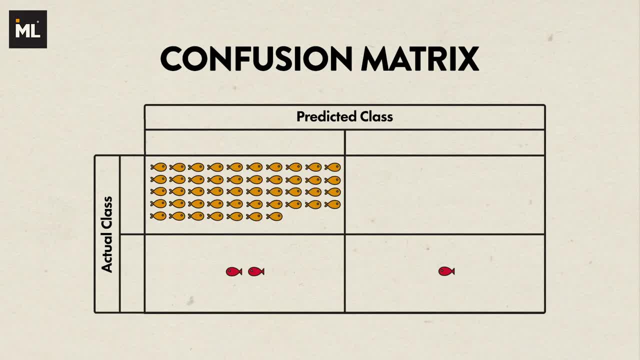 Since we only have two kinds of fish: positive class, which is the red fish, and negative class, which is the yellow fish. The top left corner contains true negative. these are the yellow fish that were correctly identified by the model. The true positive are in the bottom right corner. these are the red fish that were correctly. 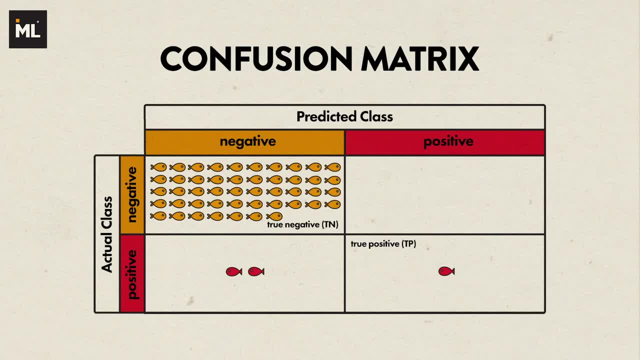 identified by the model. The bottom left corner contains the false negative. false negative are the fish that are actually red fish but predicted to be yellow fish by the model. Lastly, the top right corner contains the false positive, where the fish that are actually 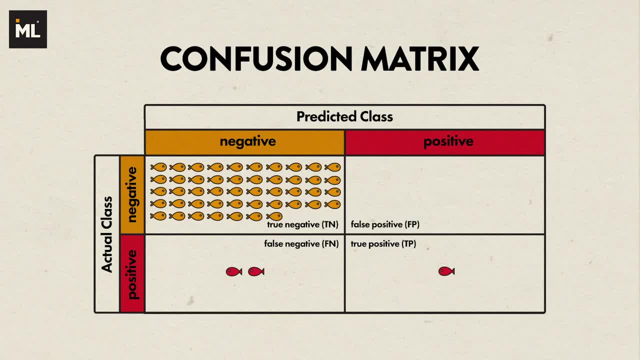 yellow, but the model thinks that they are red. In a summary, a confusion matrix clearly tells you where your model did well and where your model made mistakes. It is extremely useful for the case when the classes are very imbalanced And we are more interested in identifying positive class, in this case red fish. 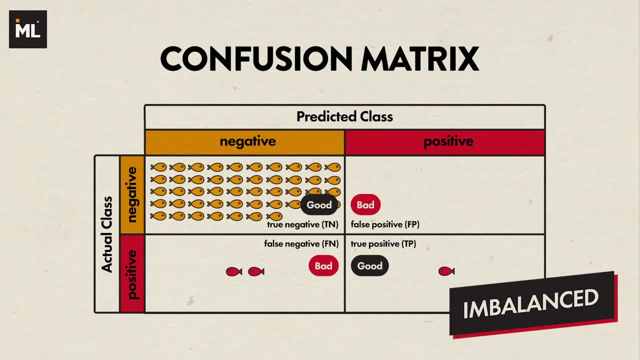 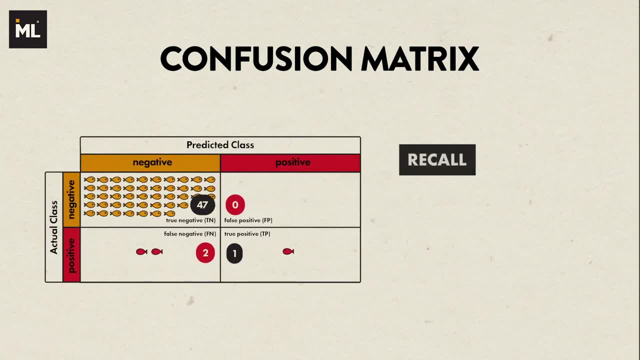 So, instead of using accuracy, we could calculate recall from the confusion matrix to measure the ability of our model to find out all the positive class. Here is the precise definition of recall: It is the number of true positives divided by the sum of the number of true positives. 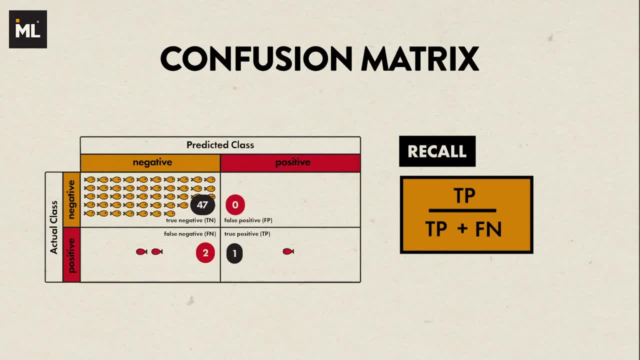 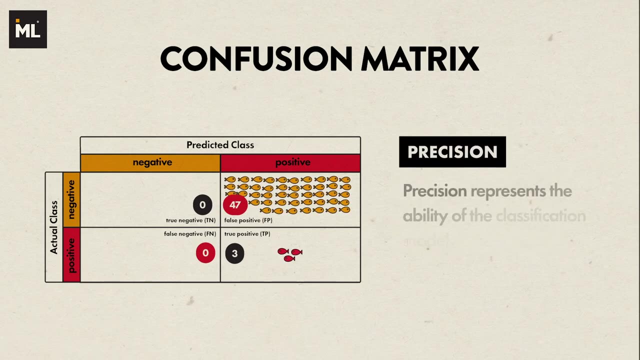 and the number of false negatives. I also want to point out that recall alone sometimes can be also misleading. If we label all the fish as red fish, then the recall simply goes to 1.. To solve this issue we need another matrix, which is precision.